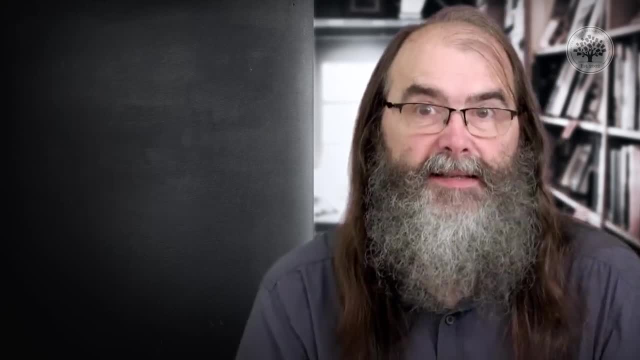 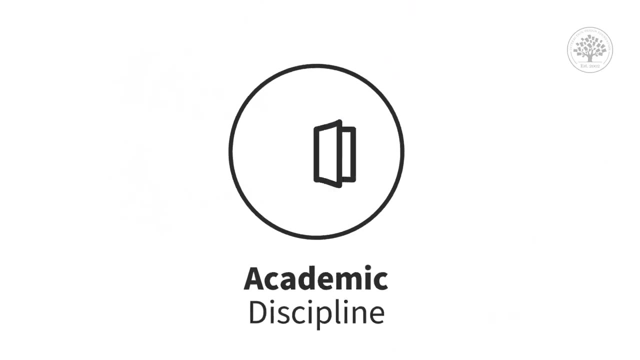 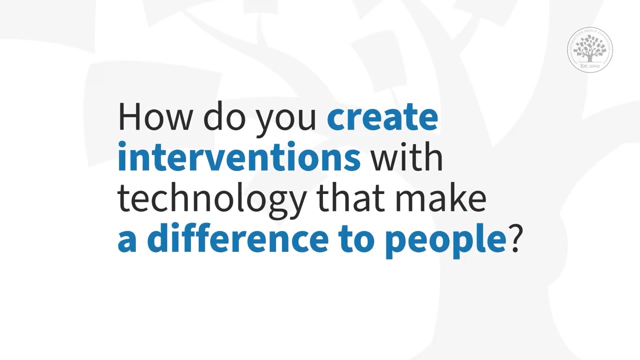 lot of you watching this video will be from a design side. You're interested in user experience design and interaction design. So one side of human-computer interaction is the academic discipline and the other is the applied design discipline, which is about how do you create interventions with technology that make a difference to people. 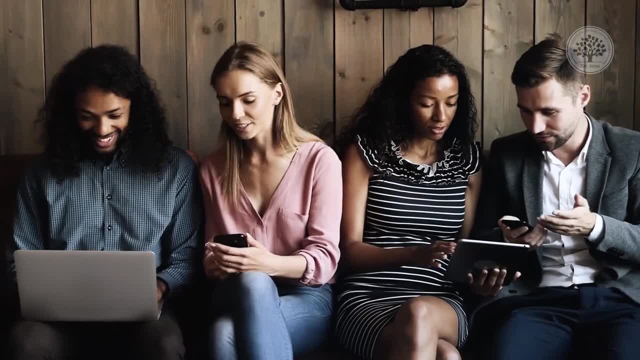 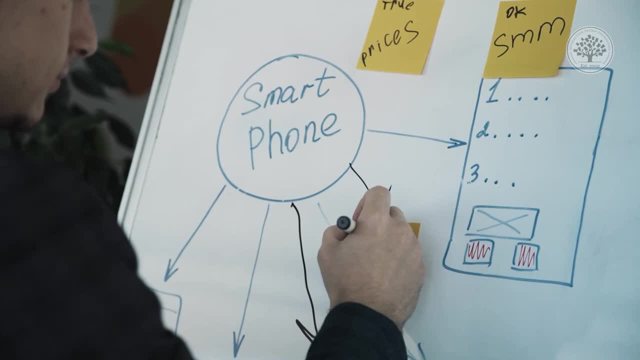 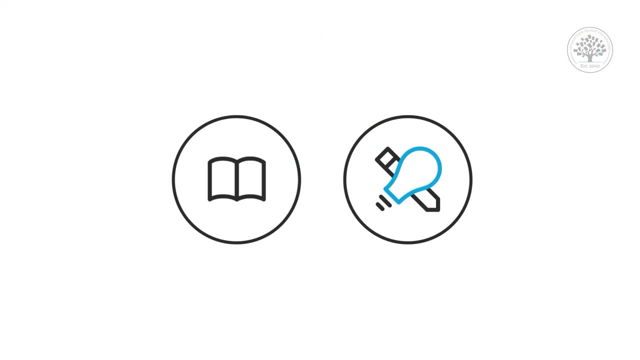 So one side is studying that computer technology and how it has an impact on people, So the way in which it works, and the other is more about saying that how do we practically change that academic study, that information we have about the way people have work, into action? 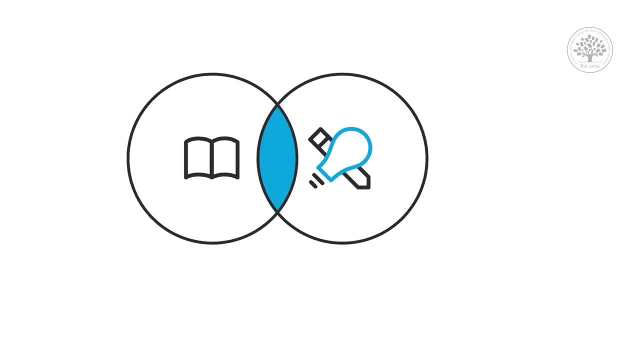 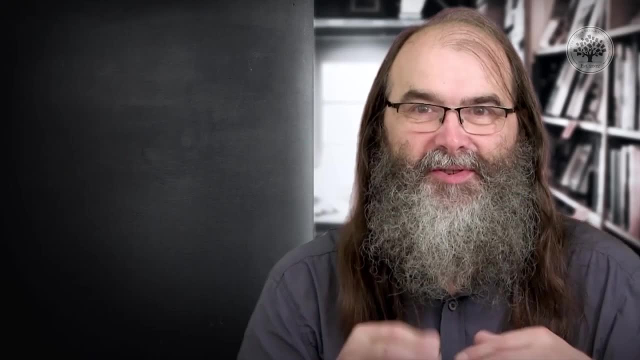 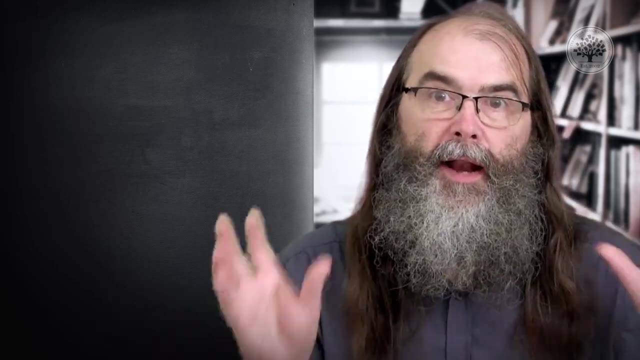 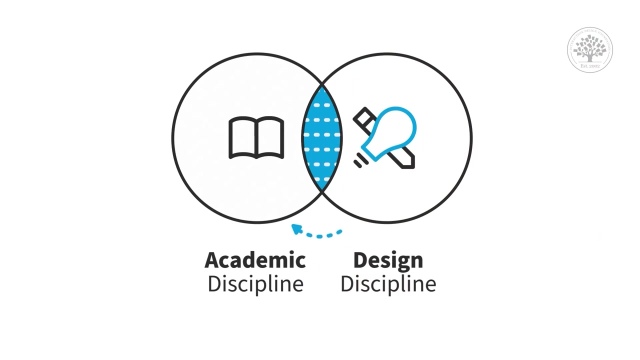 The two, of course, interact. So, on one hand, the professional experience informs the academic discipline, and you'll probably notice that I use lots of examples, some from my own experience, some from stories I know about from elsewhere, and I use those from all sorts of times in order to inform my general understanding. 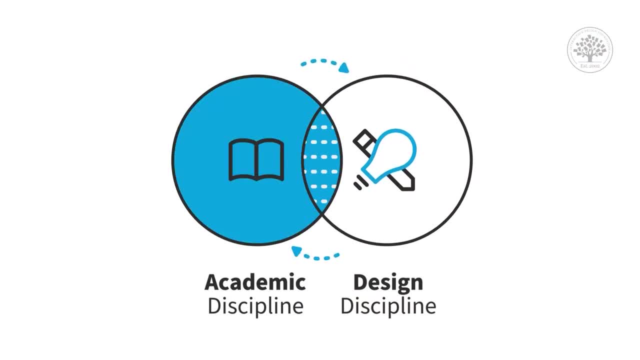 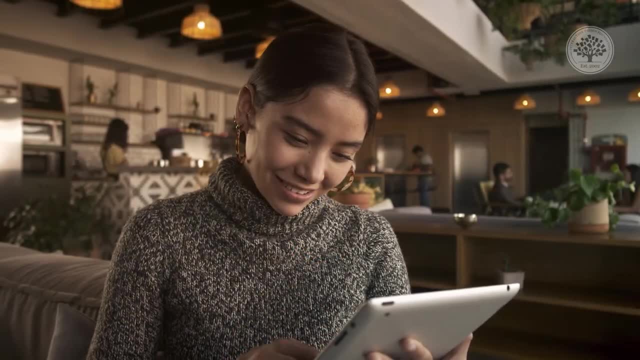 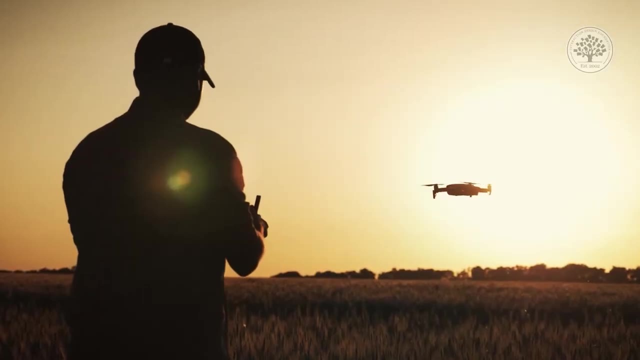 But because it works the other way around, that academic understanding, that more generic understanding, feeds back into the design discipline too. So if I understand how people interact- individual computers, how people interact together in a group when they're using technology, how people, how environments change the way people are, if those environments have technology in, then I'll 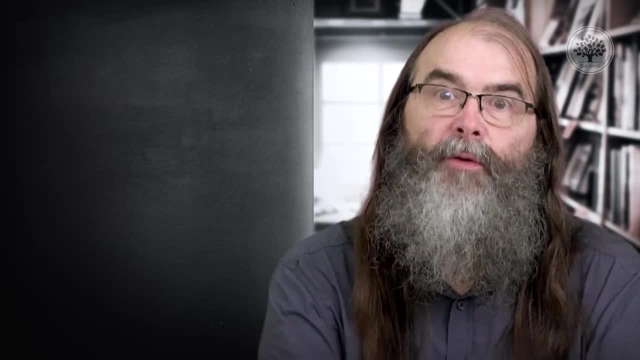 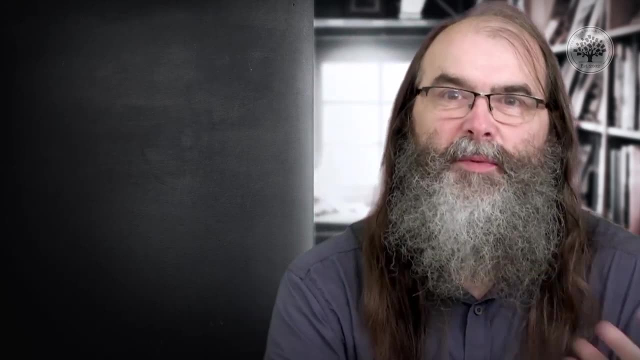 be in a better position to be able to design things effectively for them. so these two are are intermingled so within. if you want to understand human computer interaction, if you want to be part of this, you know what kind of things would I like you to know about, and so 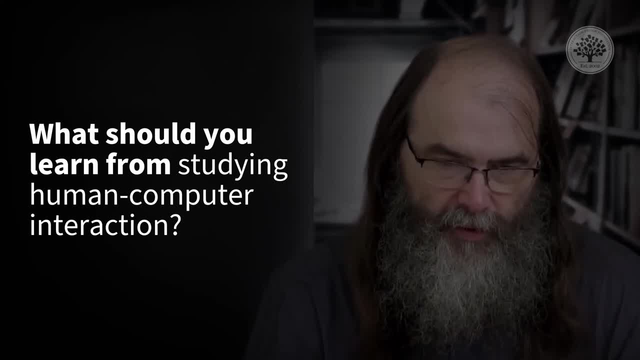 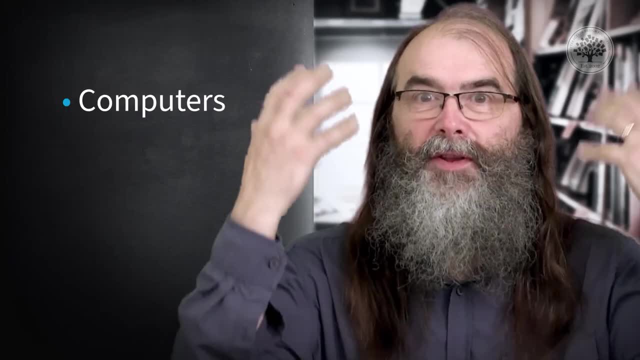 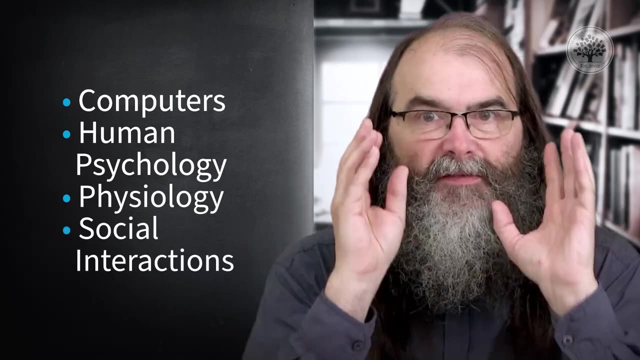 what, what, what would I hope you'd learn from studying human computer interaction? well, first of all, there's bare facts. there's facts about the, the nature of computers. there's facts about the nature of human psychology, physiology, there's a whole range of things, social interactions, and there's lots of facts about that. of course, the facts you can read in a book, and I've got 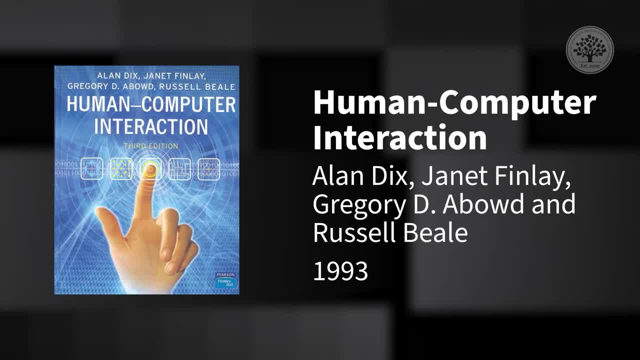 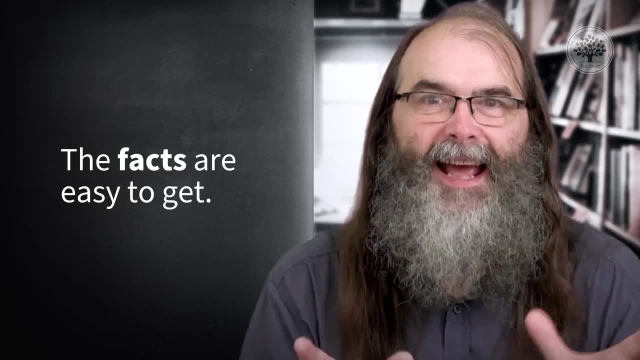 my own textbook that I produced on this and, and there are many, many others also on the web. there's vast amounts of material, so in some sense, the facts are easy to get and that you will get some of those now, hopefully, um, when I, when I talk. 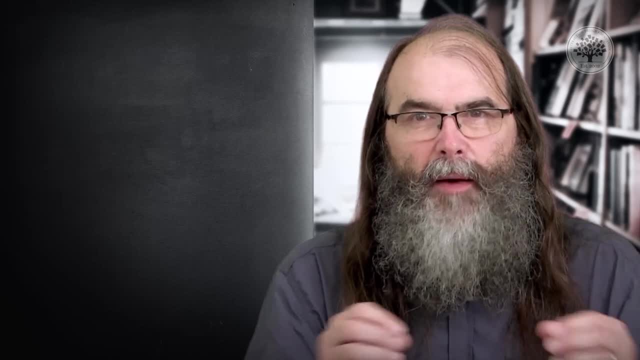 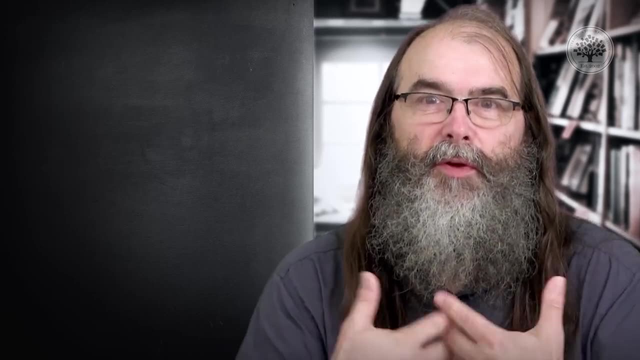 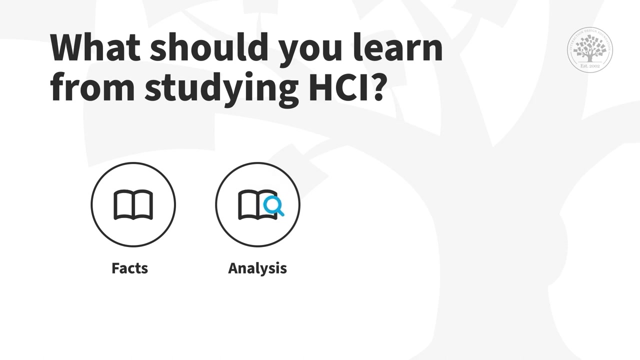 about human computer attraction. you get some of those facts. however, perhaps there's other things which are more important. um, the second thing I'd hope I'd hope you'd learn from human computer attraction is about analysis. it's about looking at a situation and trying to make sense of it. 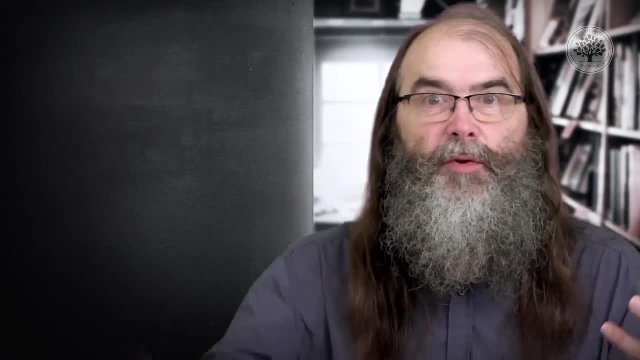 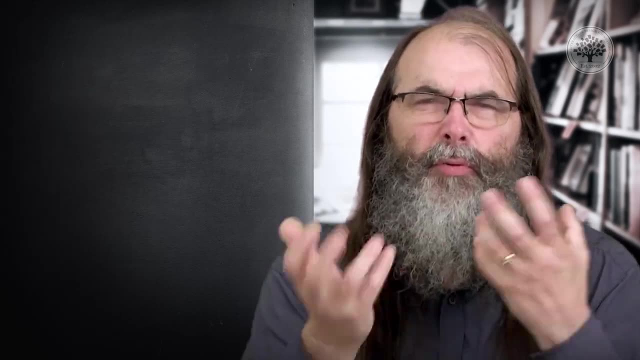 what's going on there, because if you understand the situation then you can apply the facts to the information. so it's about analysis, about picking some things apart, picking the problems that you're having a part, or picking the opportunities apart. and then, of course, once you've done that analysis, 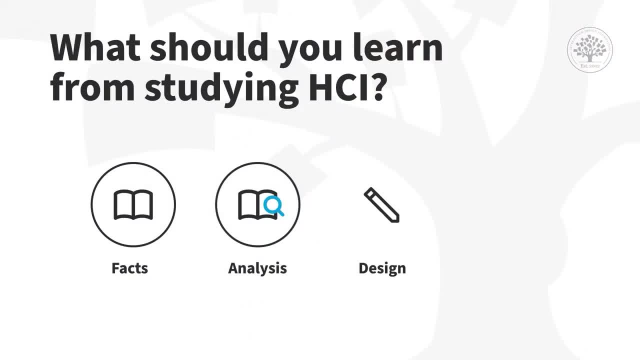 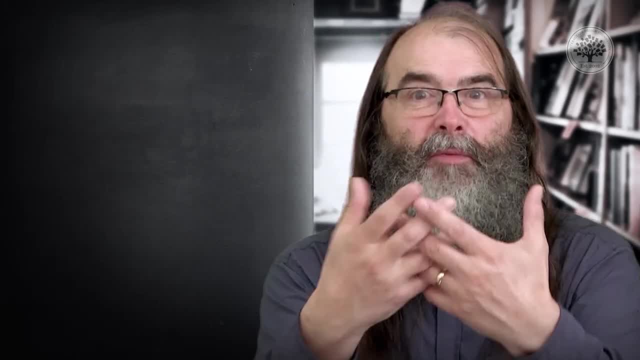 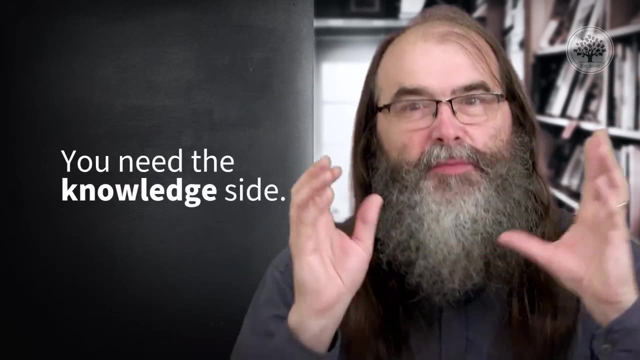 together with the facts and knowledge. from that you can then do a design job, so you can bring these things together in order to synthesize them, in order to create something that will be a solution to somebody's problem. um, but perhaps more important almost than all that, obviously you 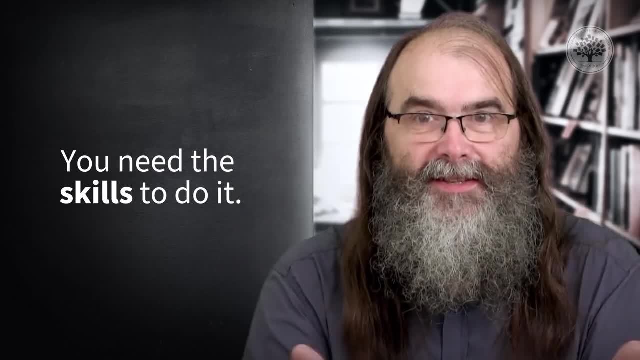 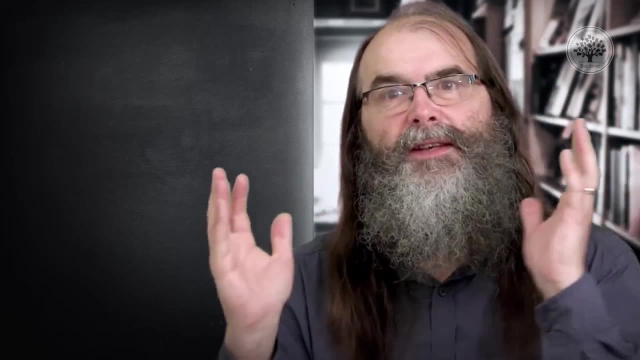 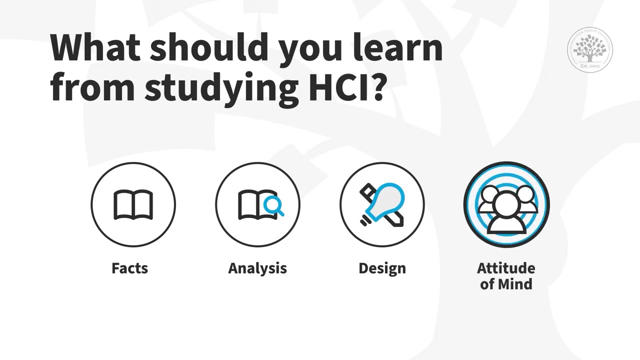 need the knowledge side and you need the skills and to do it. but perhaps the most important thing with you within human computer attraction, particularly if you think of it in terms of moving on into design, is an attitude of mine, an attitude that focuses on people, that sees real 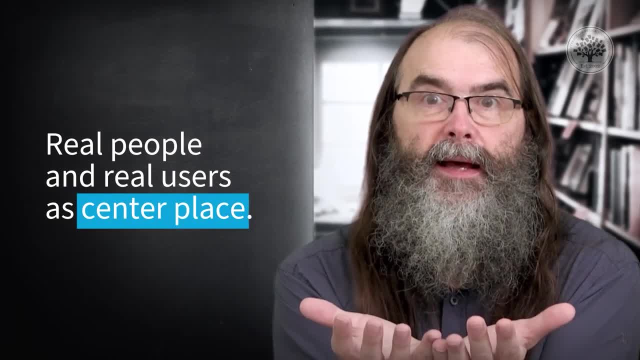 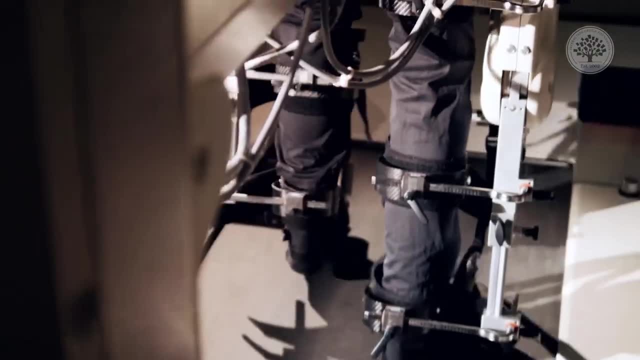 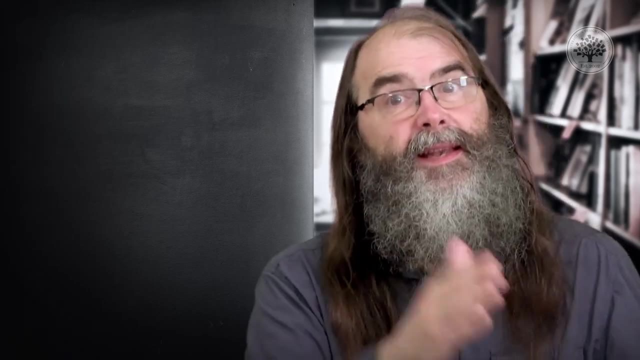 users, real situations as center place, um, that is seeking to understand people, however different they are from you, um, and to do things which are good for them, um, and make sense in their lives. so that's sort of what you know. our purpose is, in a way, particularly 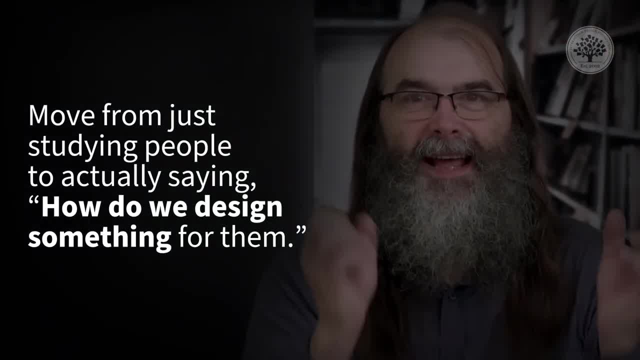 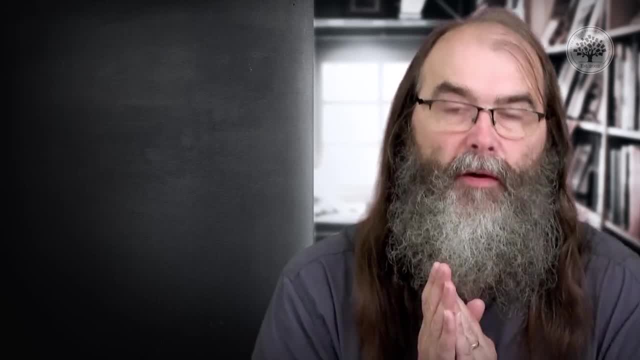 as we move from the- the sort of just studying people- to actually say how do we design something for them. so it's all kind of things. might you want to know about these and what sort of kind of things I'll often talk about in this, in this context? so one set of things is about the basics.